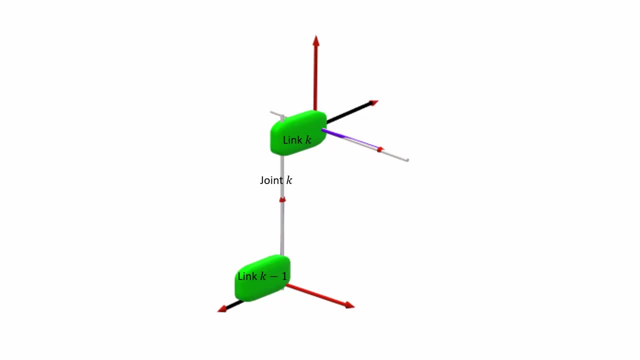 matrix between two adjacent coordinate frames, Lk-1 and Lk, in terms of kinematic parameters. Consider two links, link K-1 and link K, connected by a joint K, and also two joints, joint K and joint K plus 1, connected by link K. Two coordinate frames are assigned here, Lk-1 and Lk-1. 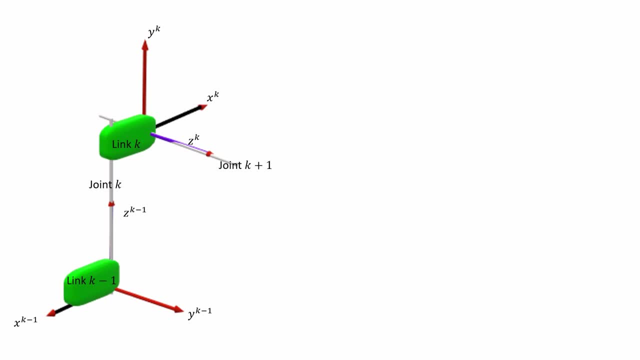 The transformation matrix between both coordinate frames can be split into four fundamental homogeneous transformations: Rotate Lk-1 about Zk-1 by theta k, Translate Lk-1 along Zk-1 by bk, Translate Lk-1 along Xk-1 by ak and rotate Lk-1 about Xk-1 by alpha k. Therefore we can write: 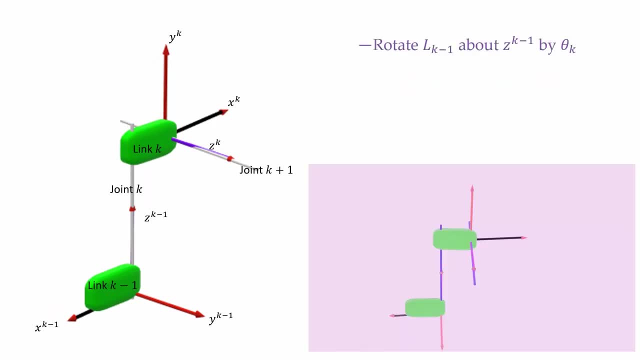 transformation matrices for each fundamental motion. Each subsequent translation and rotation are happening with respect to the moving coordinate frame axis. So the composite transformation matrix can be obtained by post multiplying each of these fundamental transformation matrices: A composite, homogeneous transformation matrix which transforms coordinates with respect to Lk to coordinate frame. Lk minus 1 is denoted by letter d, which 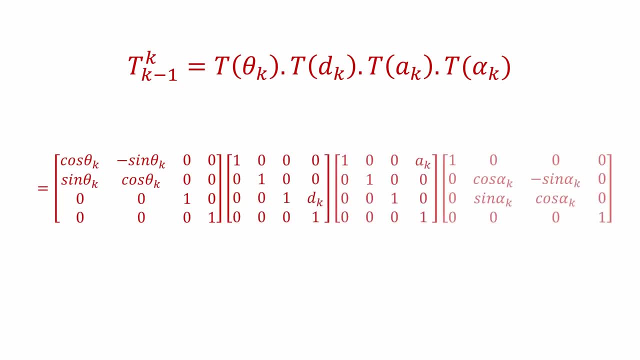 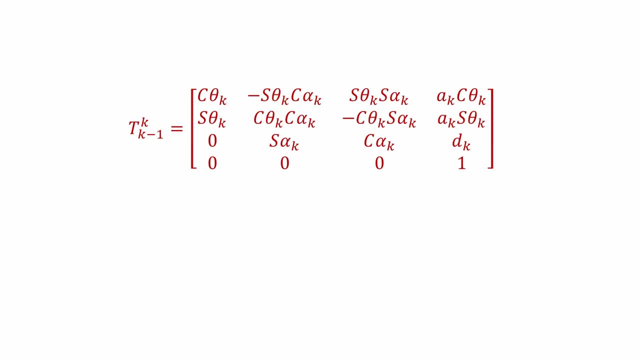 subscript being k minus 1 and superscript being k. See theta k here denotes cos, theta k. Similarly, all expressions are short. So for an n degree of freedom robot, we will assign n plus 1 coordinate frames from L0 to Ln, starting from the base frame and ending with tool coordinate frame. 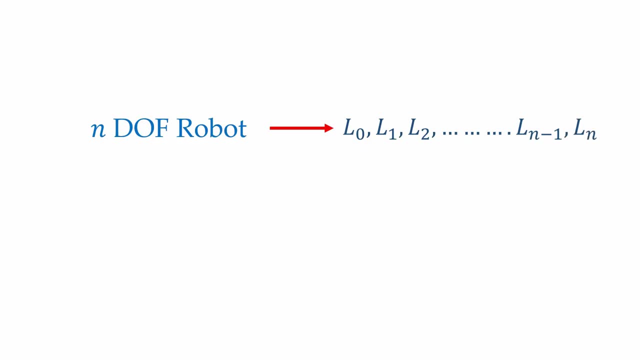 whose origin is at the tool tip. So we can find n number of transformation matrices between each of these coordinate frames. Thus we can find the composite, homogeneous transformation matrix between n- defector and base y post, multiplying each of these matrices, starting from T10 and. 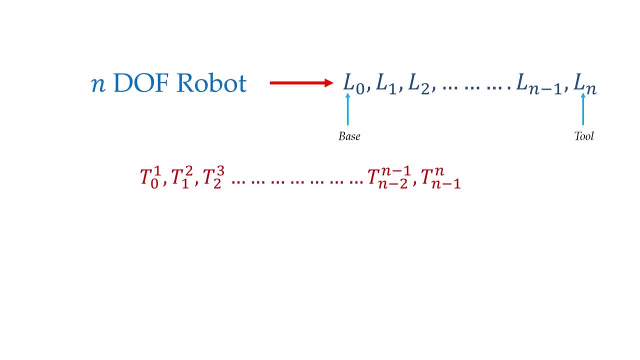 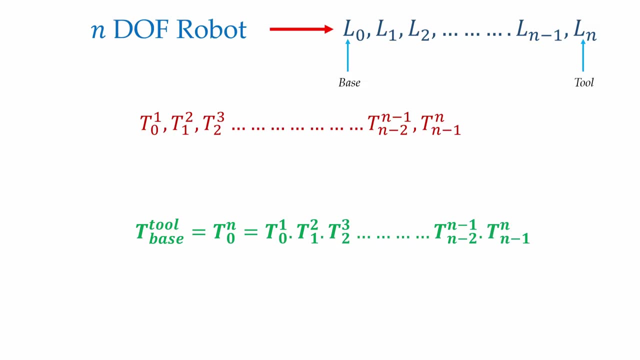 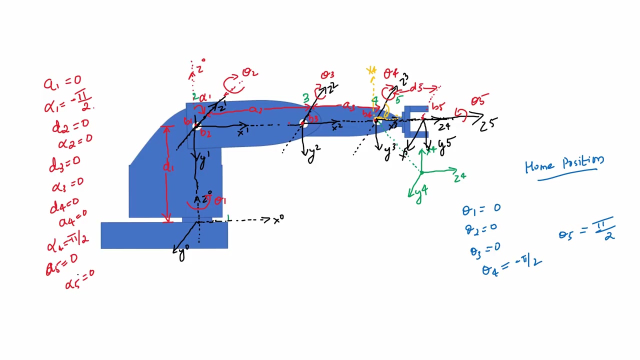 ending with Tn n minus 1.. Now let's see the example that we did in previous video. There was a 5 degree of freedom robot in which we assigned coordinate frames and identified all kinematic parameters using dynamic Hartenberg criteria. Those who didn't see the last video link is given in the description.